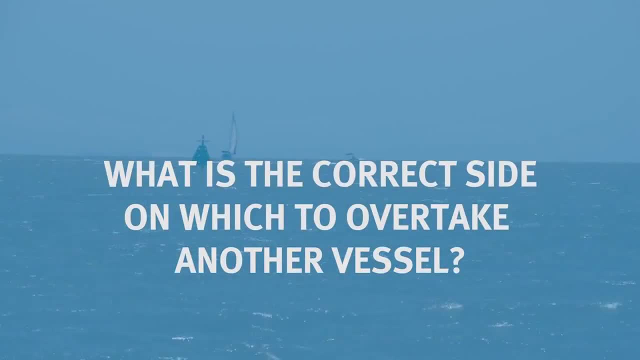 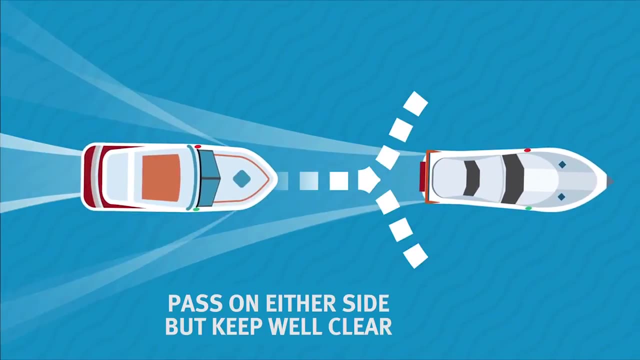 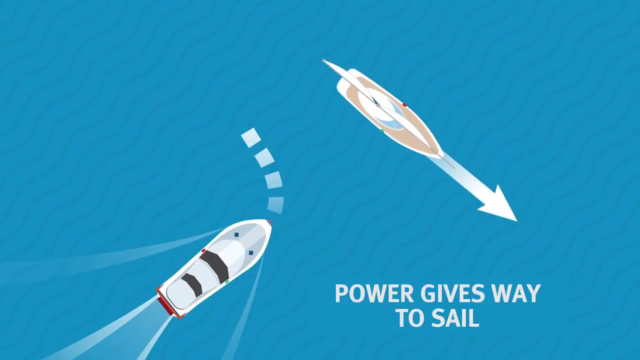 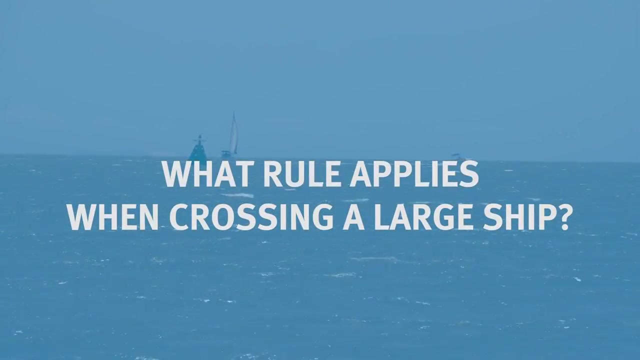 6., The 7., The 8., The 9., The 10., The 11., The 12., The 13., The 14., The 15., The 16., The 17., The 18.. 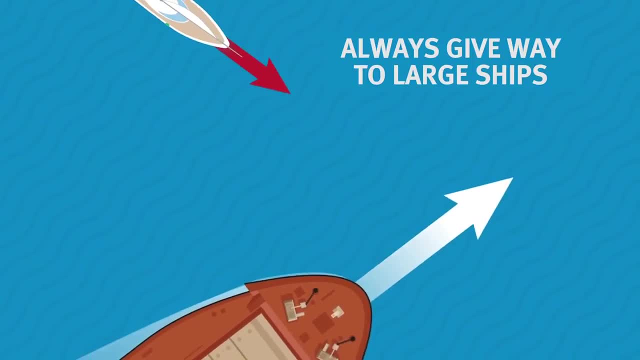 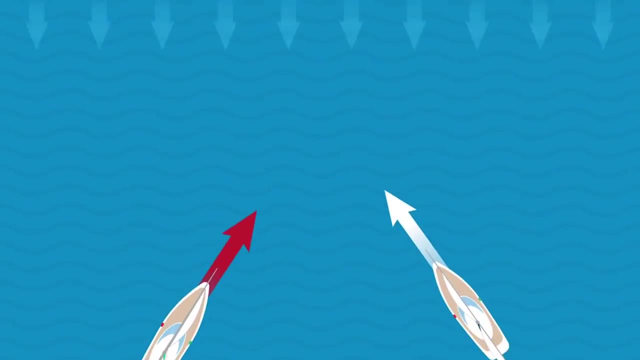 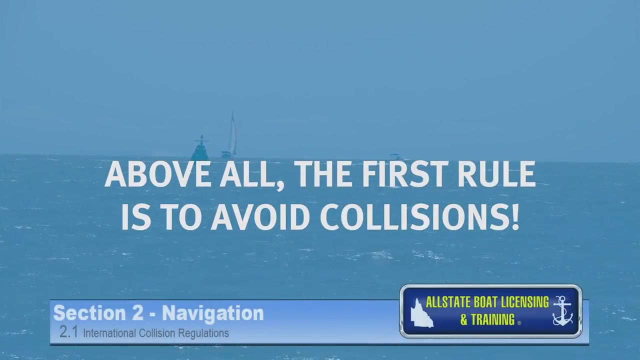 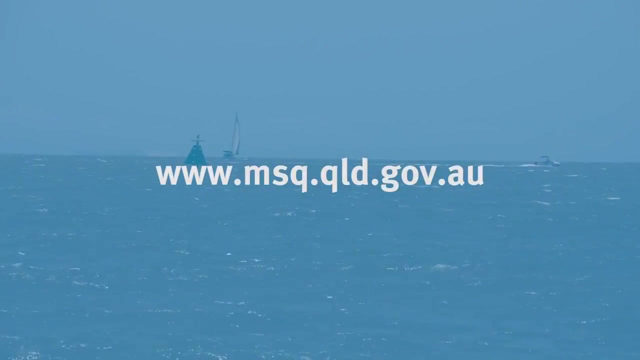 The 19., The 20., The 21., The 22., The 23., The 24., The 25., The 26., The 27., The 28., The 29., The 30., The 31.. 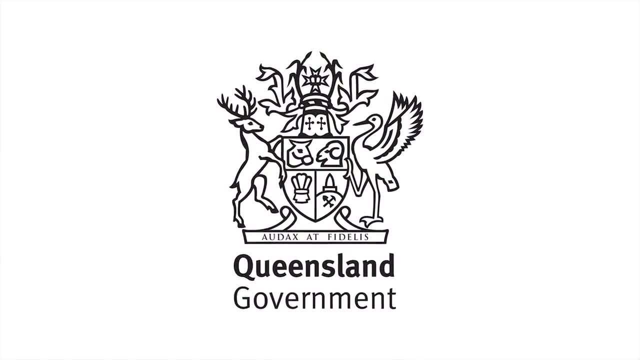 The 32., The 33., The 34., The 35., The 36., The 37., The 38., The 39., The 40., The 41., The 42., The 43., The 44.. The 45., The 46., The 47. The. 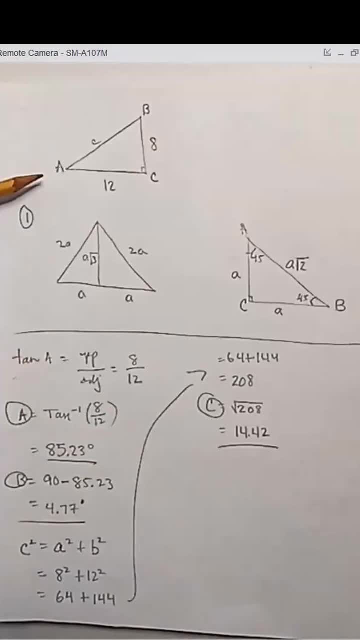 Say you wanted to solve this triangle. In order to do so you need to know how to find it. Compute the arctangent. The tangent of A equals opposite over adjacent, 8 over 12.. To get the arctangent, you take the arctangent of the tangent of A will give me A. The arctangent 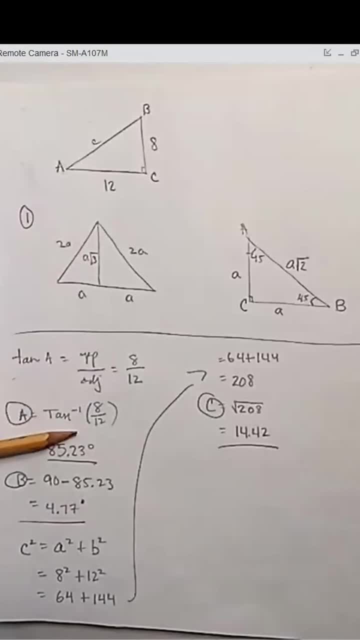 seen like this: sometimes tangent 2 to minus 1, of 8 over 12, gives you this value. So that gives you angle A. Go second tangent on your calculator to get that. Once you have this value, you can get that value because it's a right triangle. So that's one way. 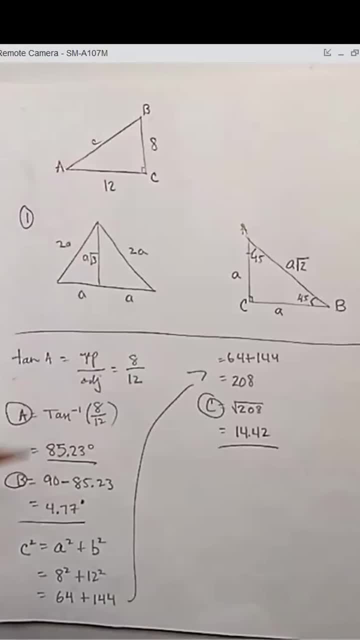 to solve for arctangent. You can find arccosangent, arcsangent in the same way. Thank you very much. 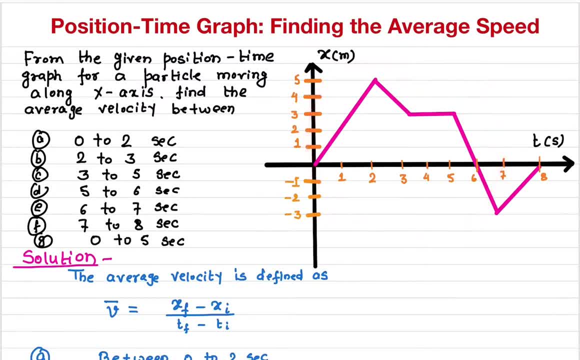 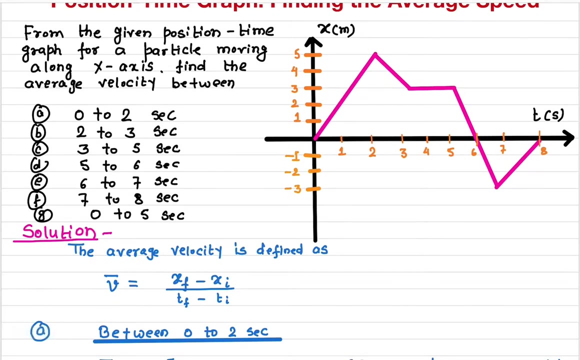 in calculating from this position time graph is: what is the average velocity between this range? What is the average velocity in this range? So, in each range, or in each time, here we have to find out the average, the velocity. So what is the average velocity? is In order to